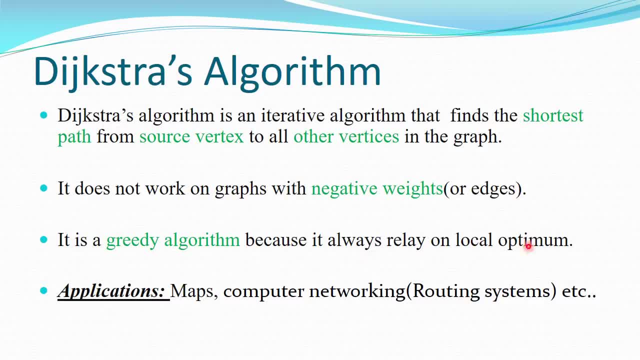 session. It's a greedy algorithm because it always relies on local optimum. So every iteration, if you look at it, always relies on local optimum solution. So application maps. So in a practical case, if you want to go from one place to another place, you can see you can come across various 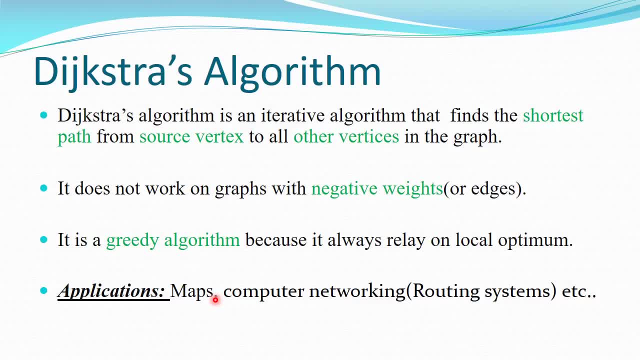 paths. So using this algorithm we can choose the shortest path among them. Computer networking, so you know routing system right. So when you send a packet from one computer to other computer, so there could be many number of paths. So we can use this algorithm to find the shortest path. 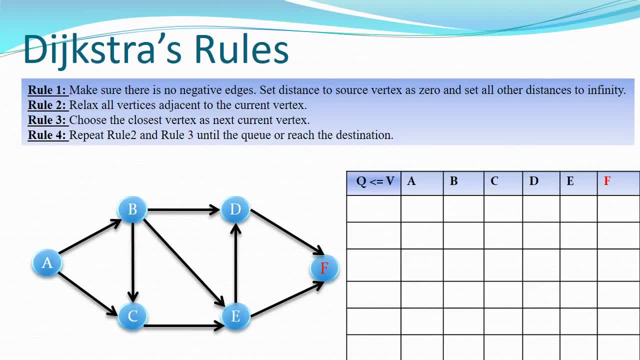 among them. Next, in this slide we are going to see what are the major thumb rules for Dijkstra's algorithm, And then we'll try to apply those rules into this animation and we'll try to visualize that as well. First, let us start with the rules. Rule one: make sure there is no negative weight. 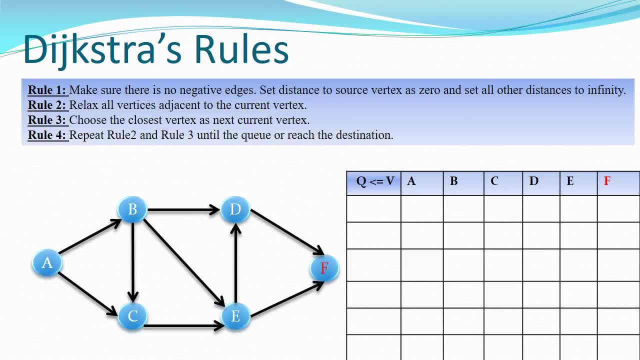 change. Make sure there is no negative weight change. Make sure there is no negative weight change. So we have to make sure there is no negative edges in our graph. So if you look at the edges, which are weights which I chose, all are positive edges. If you look at any edges or weight among, 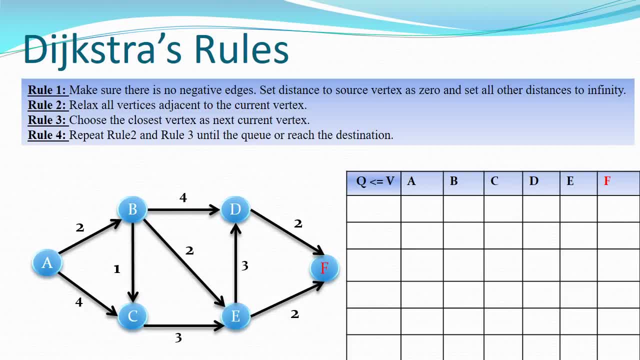 the vertex, vertices or nodes, you can see all are positive edges. Then actually, if you want to do any search or any path, on any path, actually, you have to choose first starting and final vertex. So let us choose A as our starting vertex and F as our final vertex. So our goal is to find the shortest. 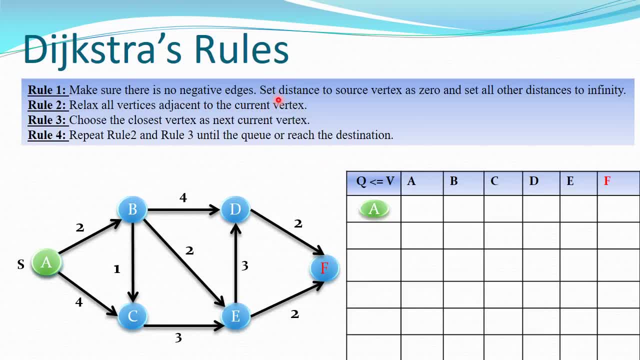 path from A to F. So next, set distance to source vertex as 0 and set all other distance to infinity. So what does it mean is first, so we are choosing the distance to source vertex as 0 because it is actually self-directing distance. 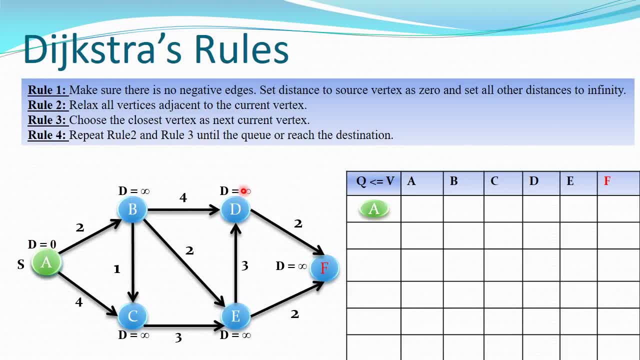 is by default 0 and other all vertices. if you look at, I put it as infinite because we haven't explored it yet. so there is no, you know, path value we have from here to any other nodes. so if you look at right side, we have tabular. 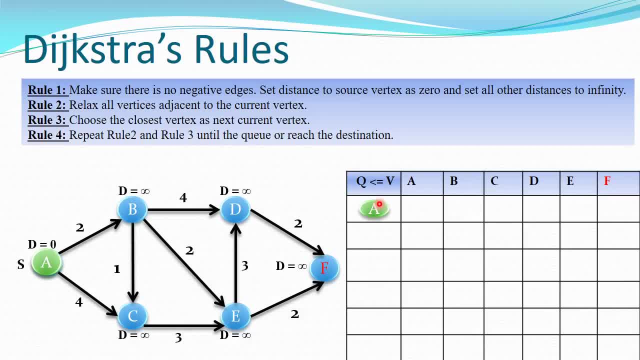 columns- here you can see we have actually left side. we represent it as current vertex. basically, when we do every iteration we will keep the current vertex in this column and these are all the possible adjacent vertices. so we will every row basically represent a complete iteration from a. 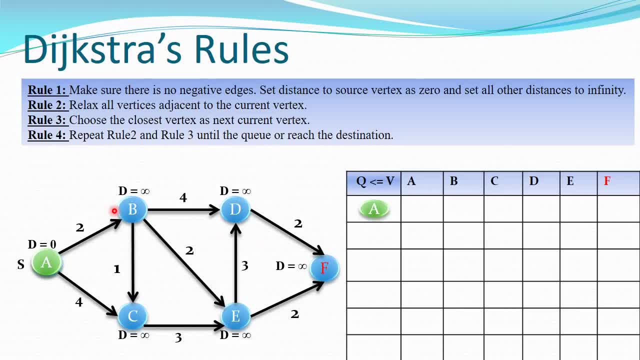 particular current vertex. so so let us start with now rules. so let us start with now rules. rule 2: relax all vertices adjacent to the current vertex. so if you look at the adjacent vertices first, from starting vertex or current vertex, you can see B and C are the adjacent vertices for A. so we have to relax these. 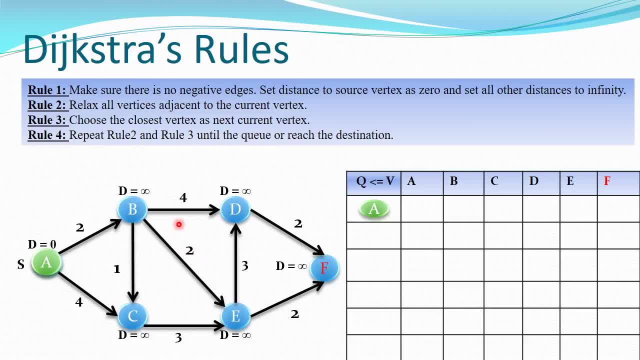 things. so basically, first, for that there is a you know rule and also we have actually the tabular column. we have to fill it. so first what you have to do, first times into the iteration A to A: by default I'm keeping as zero, because that's what it is. A to B: we have one adjacent and A. 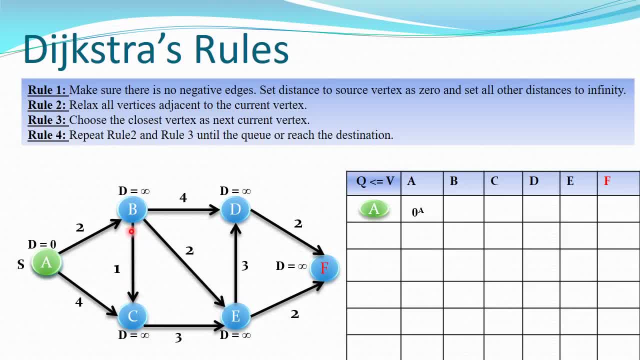 to C two we have right. so for these two we have to apply the rule like this: if distance of current vertex plus distance of adjacent edge is lesser than distance of adjacent vertex, then what we should do, we should update adjacent distance with the new shortest path. so that means that here current 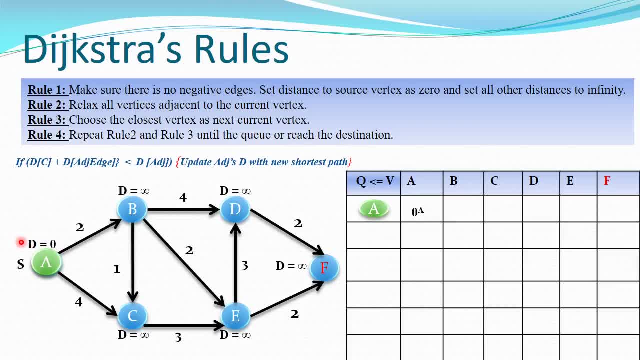 vertex is a. so here, actually initial distance, we have 0 and plus 2. this is what the adjacent edge weight. so 0 plus 2 is 2. so basically this is lesser than the distance which holder in this adjacent vertex, so it is infinite. so 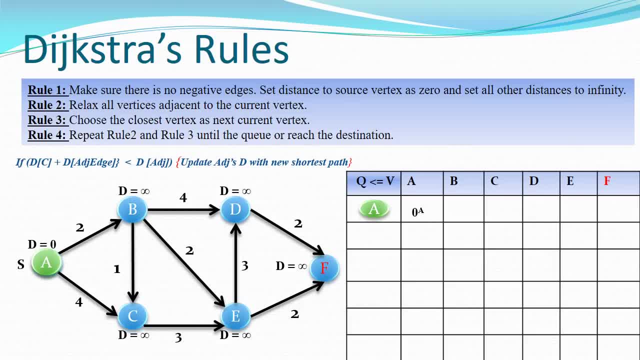 what we can do. we can basically relax this one. so what we do, we just update that into this descent. so here, look here: a to b: I mean we are just representing like 2, and on the top we have mentioned 8. so that means that from a to be, that's. 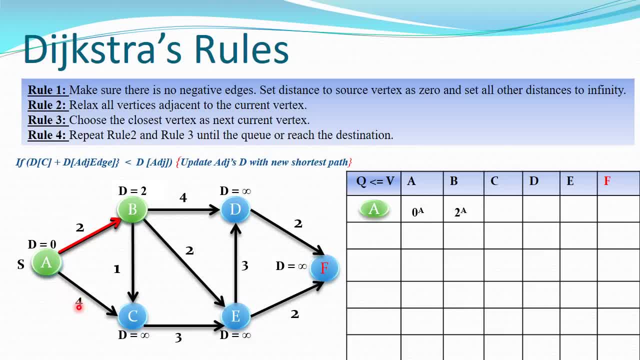 what it mean, okay, so next we have one more adjacent vertex for from view, so let us visit that as well. so if you compute that relaxing formula, then you can see again: D is equal to 0, 0 plus 4 is 4 less than infinite. so we can, what we can do, we can, you know, update this as 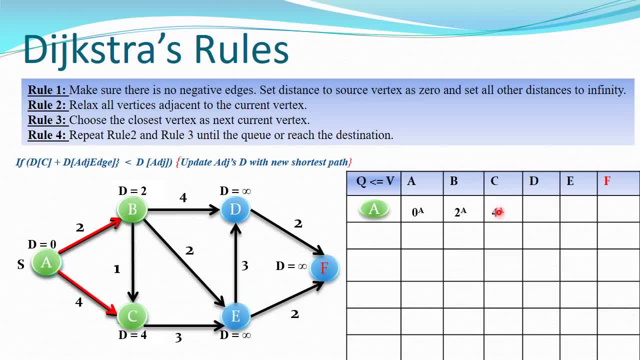 well. so we have put here also: A2C is 4, so next we don't have any other adjacent vertices right from here. so that's what we have: to see what next current vertex we can choose. I mean with next. so for that the rule 3 says: choose the closest. 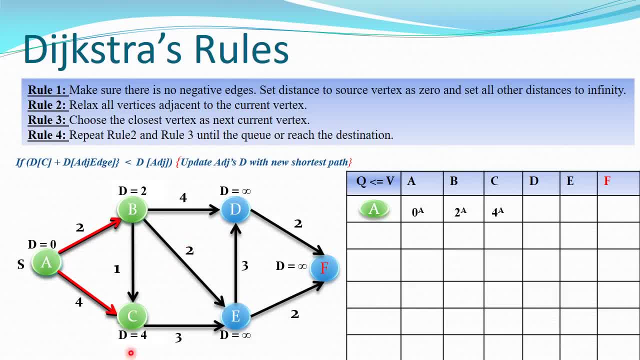 vertex as next current vertex. so if you see, among these two vertices which we calculated, you can see B as a shortest path, one. so what we do? so we have to choose this B as our next current vertex. so before we go for it, because we have to just make sure, because A to D we don't have any paths, so we put this. 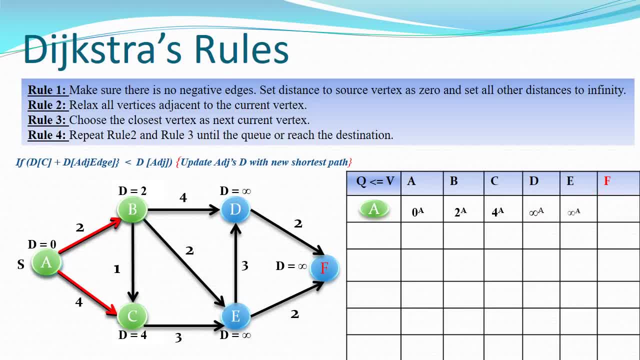 infinite A to E. we don't have, so we put it as infinite even. same for F as well. so first iteration: we have done all those things. then we have chosen B as the shortest path, and then we have to choose B as the shortest path, and then we 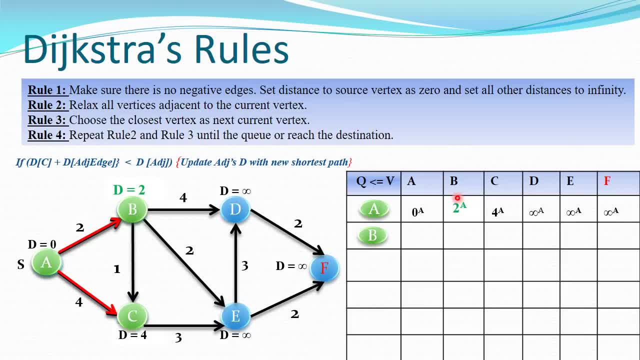 as our next current vertex, so big. now this i just put it in green color, i mean that there is no further processing one, this is actually finalized. so next, we have chose, chosen b as our next current vertex. right, so now let us iterate on the adjacent vertices. so b has three adjacent 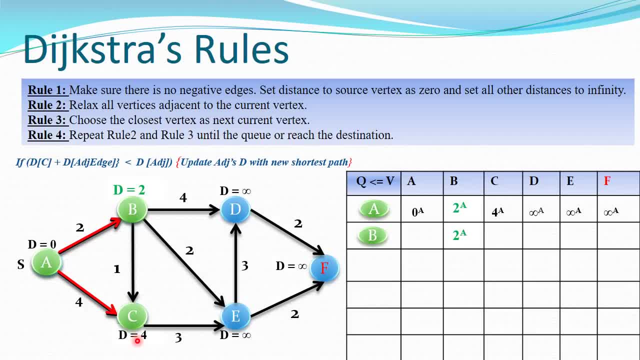 vertices d, e, c: right, so let us start from c. so so again you apply the rule. so here the current vertex is b. b is equal to 2, 2 plus 1 is 3, 3 is less than less than 4. so i think so as per rule. 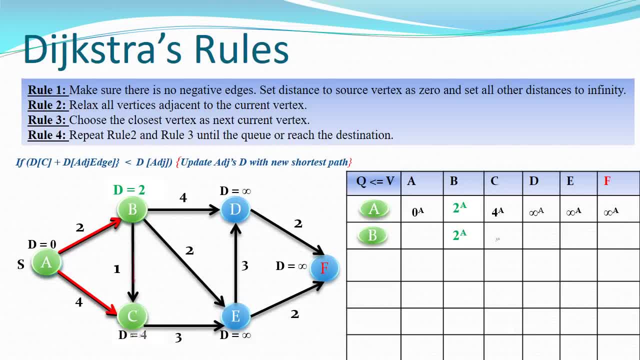 we can update this distance to 3, so let us update that. so we updated 3. so now b, 2, c is now basically 3, distance is 3.. so by the path, if you look at from c, if you want to go to a, c to b and b to a, so that's what it says. and then we have two adjacent vertices again. 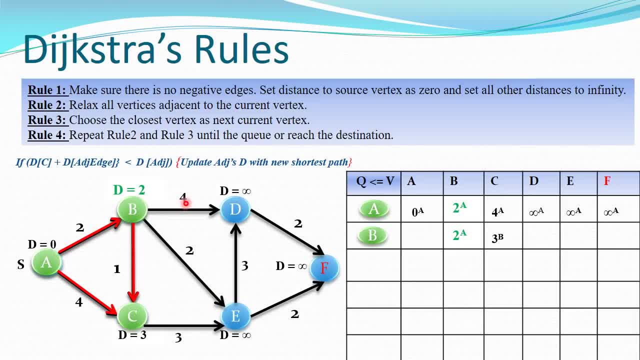 d and e. so if you look at here, 2 plus 4 is 6. it is lesser than infinite. so we can update here also: 2 plus 2 it is 4. again, we can update these two vertices with the current calculated distance. so now, if you look at, 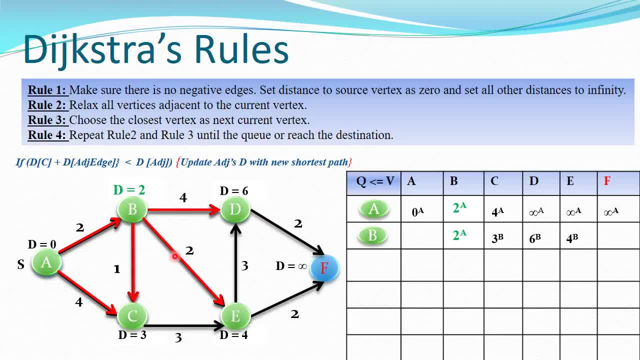 six and four we have updated and then now there is no more further vertices to visit, so we just put other all as essential. so i mean to say whatever was there in the previous value, just we keep that here also. so now we have to choose again which is the shortest one from this list. 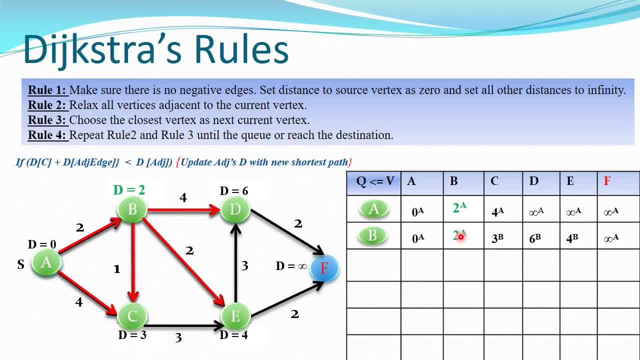 so already we have chosen two, i mean b, so here we can't go now. so rest of the thing, we have three, six, four, so among this three is the smallest one. so basically this is from c, part c. so we'll go to three and c and we will choose that as our next current vertex. 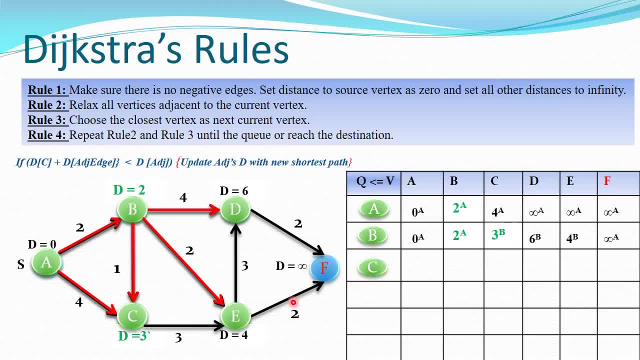 so we have chosen c as our next current vertex. so from c, if you look at, there is only one adjacent vertex. so, as per rule two, we just try to relax that. so when we play the rule 3 plus 3, 6. so that is basically. 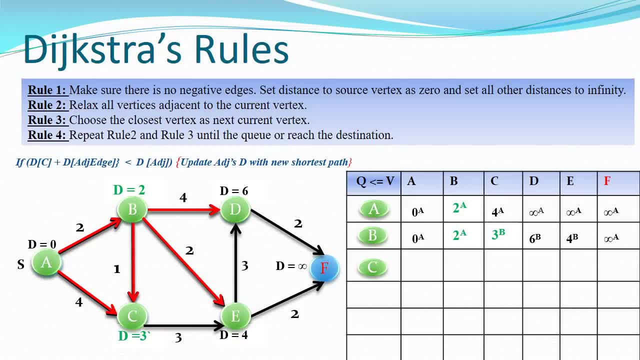 bigger than 4. so we cannot be no need to, you know, update that. so what we'll do, we'll keep the same. so we'll keep the same. and next, we don't have any other adjacent vertices, so we will just put all the existing values into this new, this row. so now again. next we have to choose the. 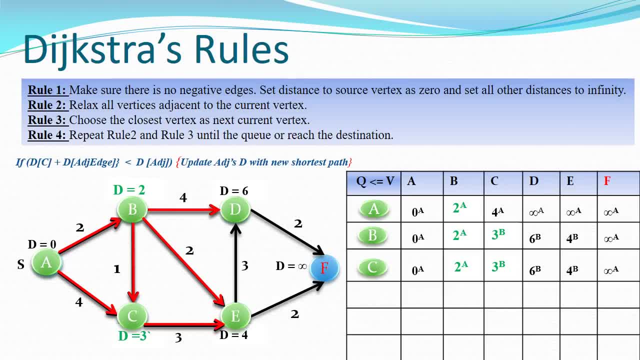 shortest smallest value. so i think between six and four, we can choose four as our next shortest one. so here then, our next current vertex will be e. so from here again, we'll apply the rule to relax all vertices. so it has two adjacent vertices. so so let us relax one by one. so so, if you look at, 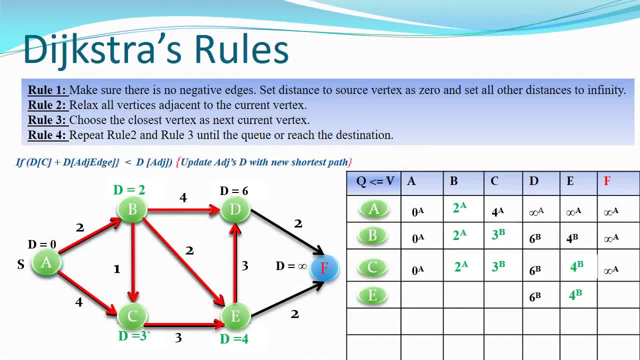 so here it is three. four plus three is seven. so we are not updating that, so we are just keeping the same. and here, if you look at four, four plus two, it is actually six. so it is lesser than infinite. so we can update that. so we have now three f we. 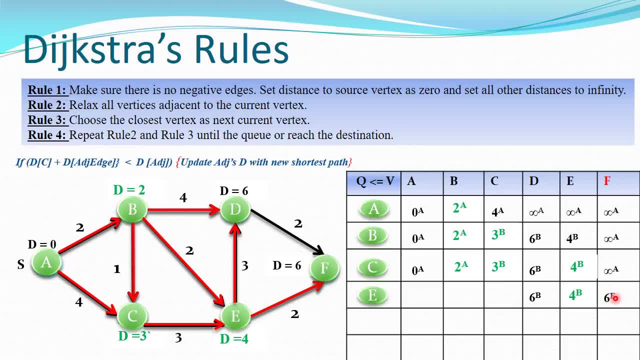 have six as a path. you know distance, so now that's all it has. so now we can, you know, uh- copy rest of the things into the new. this is current row. so we did it, and now again we have to choose the next shortest one. so we have two vertex, or you know? 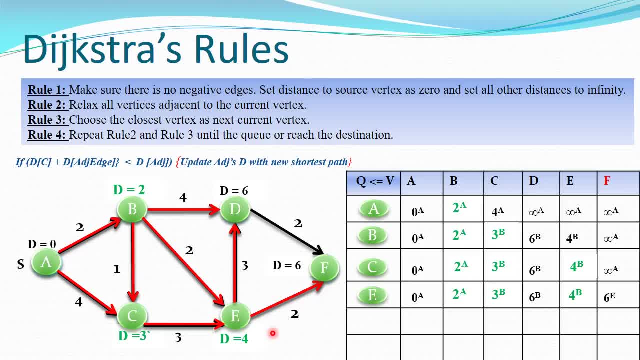 we have to keep the same value so we can choose the first one. so if you look at the six, let us choose six as our next one. so if you look at from six, so from d, if you look at six plus two, six plus two will be eight. so eight is basically bigger than whatever we have holds. 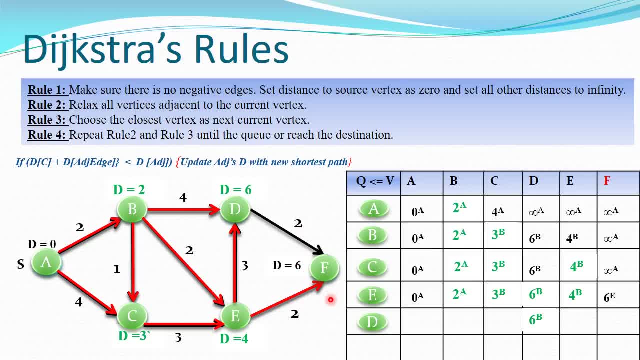 already, so its condition is fail so we don't need to update that. so what we can do, we can keep the same value. so we are keeping the same value here and the rest we just copy. as usual we do, we copied all those things. the final thing is actually we have in our thing is like six. 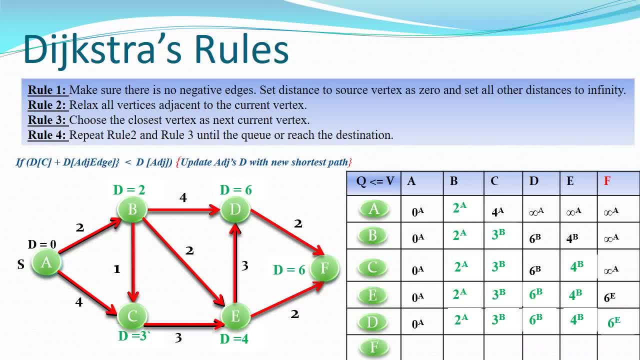 yeah, this is what depending. so, if you from, if you, we can choose that as our next vertex, current vertex. so from there, if you see, there is no further vertices so we can now choose. we can just copy all those things from the existing tool. so if you look at, this is our final, you know, shortest path value. 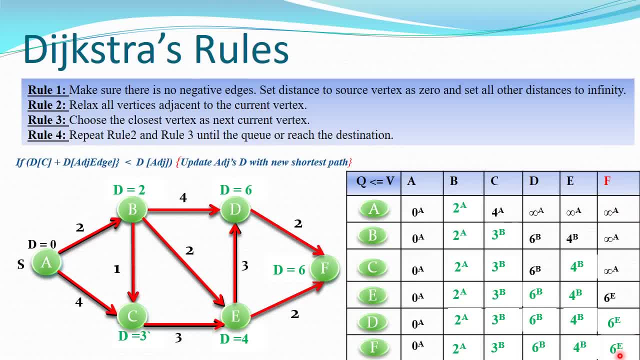 here actually from f. what is the shortest as we look at six right, so shortest part from, but the path it is to from where it comes: e. so if you go to e, it is actually it says from b. so if you go to b, that will be r. you know it is from a, so that is what actually it says. 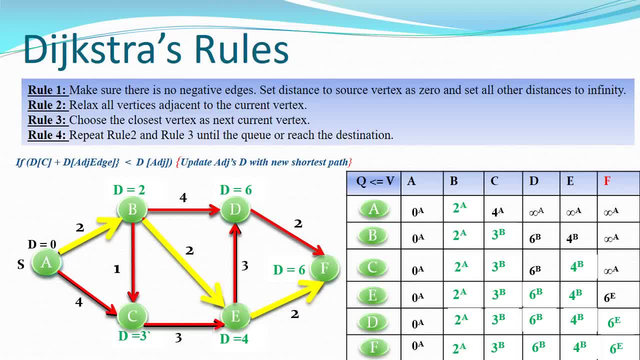 shortest part. if you look at in our diagram, it will be something like this. so this is what i said. so from f you'll go to e, right from you have to e, and from e to b. so e to b and b to a. so basically we have visited all the. 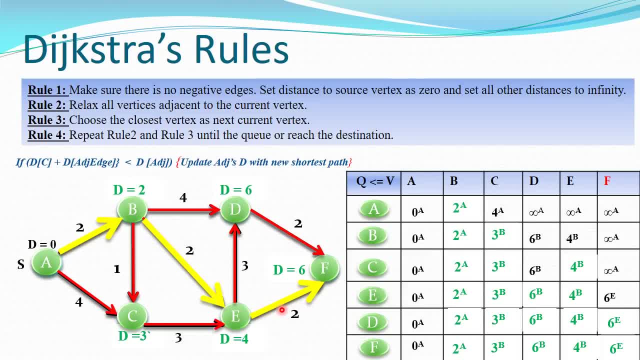 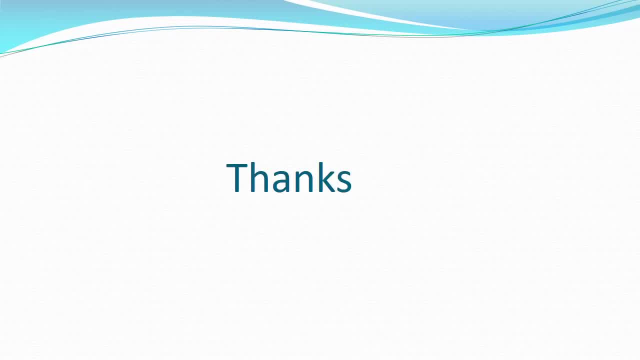 values and we found all the shortest path on this particular graph. that's all we have for today. thank you for watching. please do like it if it was useful. thank you.